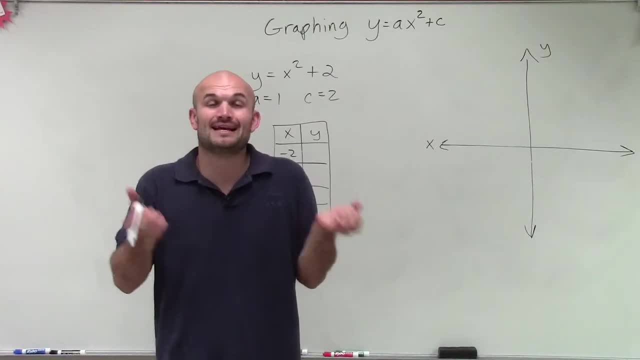 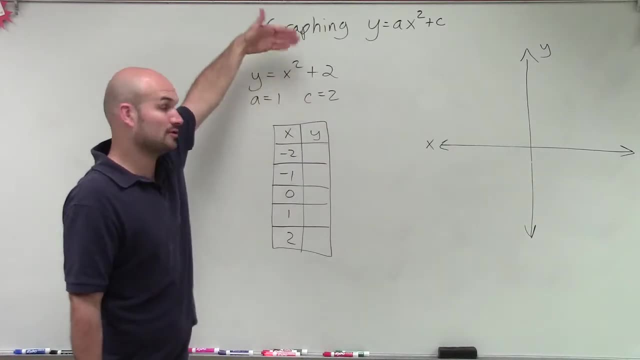 remember to graph our parabola. a parabola is a set of points that has an x coordinate and a y coordinate. So if I choose my x coordinate, I need to figure out then what is the y coordinate. then that is a part of this parabola, or this? 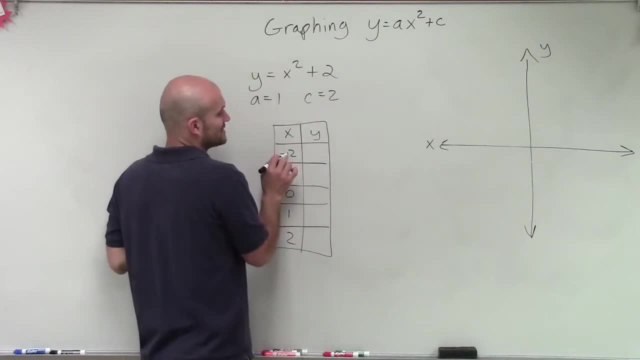 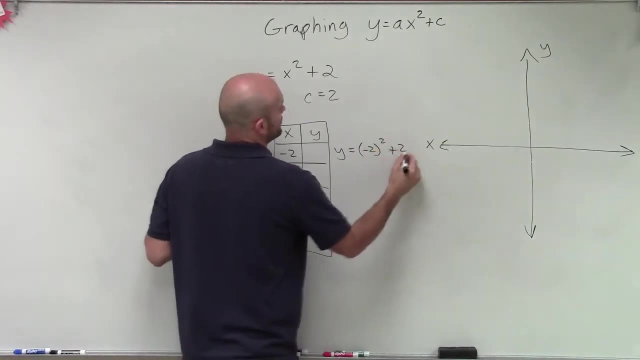 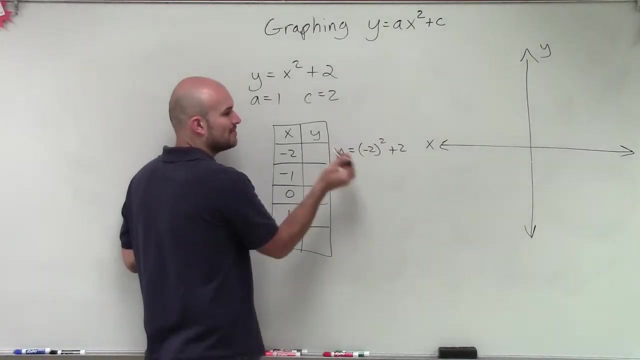 quadratic. So to do that I need to plug these x coordinates in into my equation to find the y value. So I have: y equals negative 2 squared plus 2.. Now notice my use of parentheses. I'm putting parentheses around this when I square it, because I'm not doing 2 squared and then multiplying by. 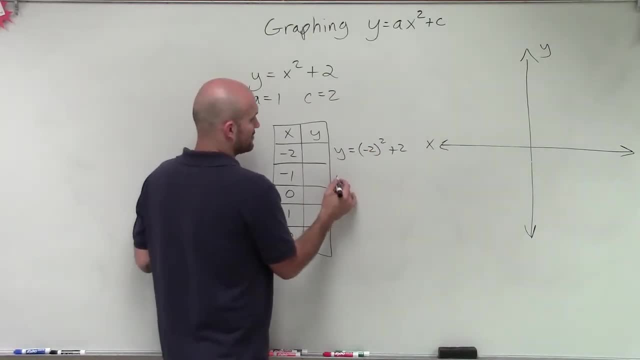 negative 2.. I'm actually squaring negative 2 squared, And what's really important about that is well, the squaring function is always going to make it positive right. So therefore, you can tell that it doesn't matter if the number that I square is going to be positive or negative. 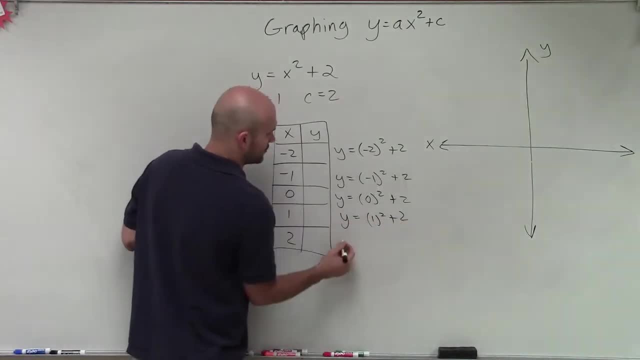 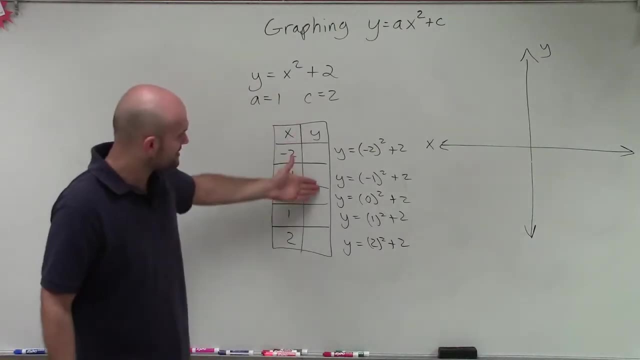 It's still going to give me my exact same value, And that's what's so cool about this- Really really cool, right? What's so cool about this is because now, when I go into this, I know that, to the left and to the right, the squaring- it doesn't matter if I square the negative or the positive. 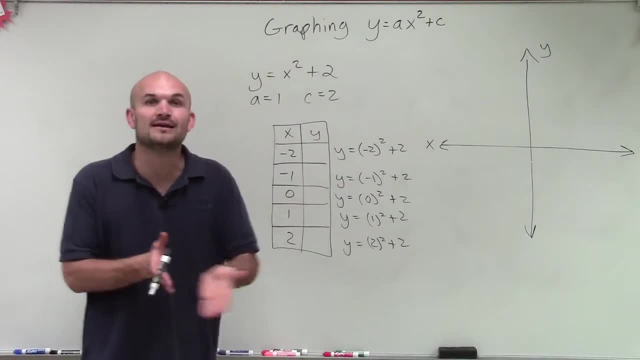 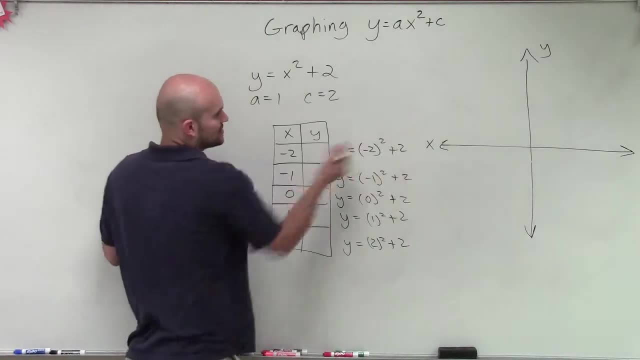 I'm going to get the exact same hour And that's the important part about that axis of symmetry, right, Remember, the axis of symmetry is your symmetry of your graph. The left side is equal to that right side. It cuts the graph in half. So let's go and evaluate our answers. So I have negative 2. 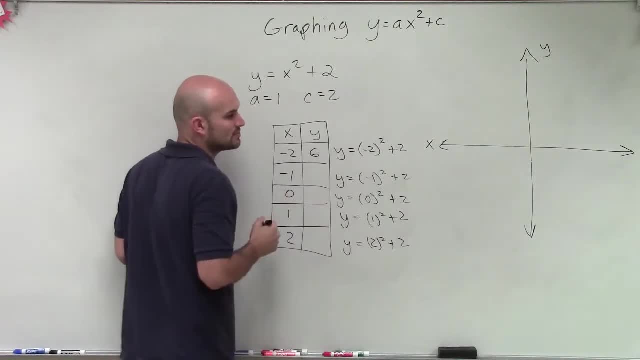 squared is 4, plus 2 is 6.. Here I have negative: 1 squared is 1, plus 2 is 3.. 0 squared is 0, plus 2 is 2.. 1 squared is 1, plus 2 is 3.. And 2 squared is 4, plus 2 is 6.. So you can see that. 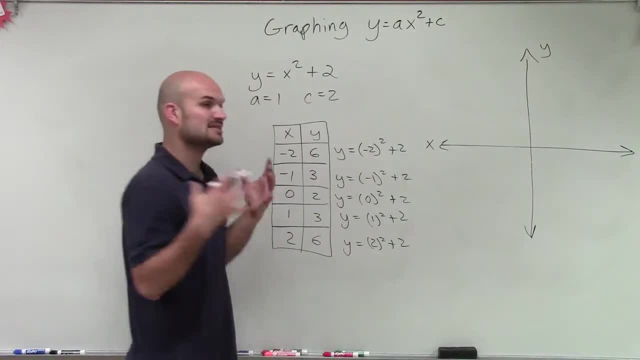 it's symmetrical about. our axis of symmetry is at 0.. Now let's plot these points and let's see why is it that the axis of symmetry is at 0.. So I have two points: negative 1 and negative 2,. 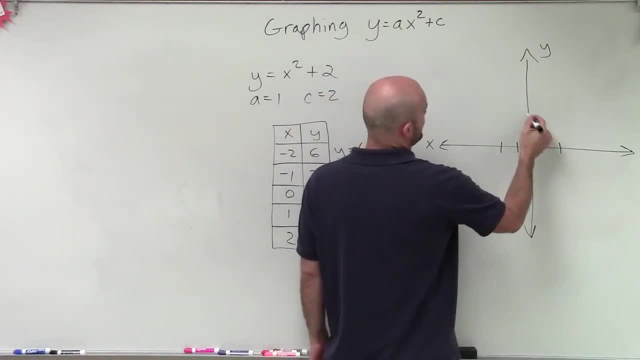 positive 1 and positive 2.. And I'm going to go all the way up to 6.. 1,, 2,, 3,, 4, 5, 6.. So I go up to negative 2, positive 6,. 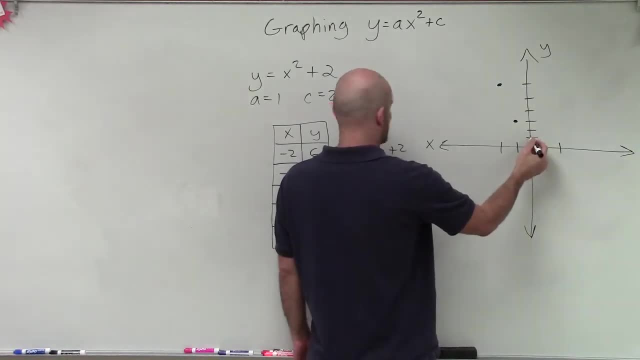 negative 1, positive 3, 0,, 2, over 1, up 3, and over 2, up to 6.. So when I graph my parabola here, notice that the graph is going to continue in this upward direction And you can see. 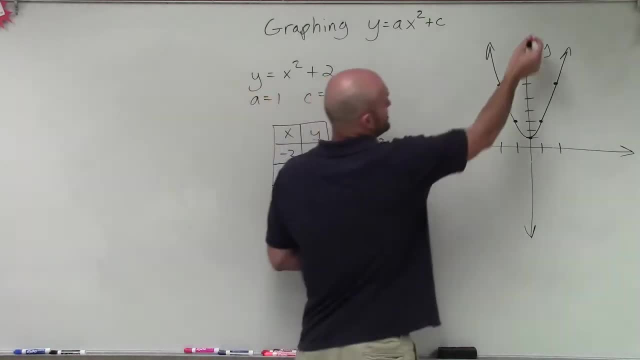 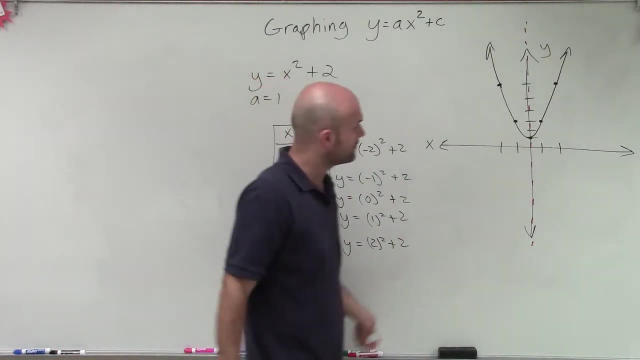 that this dotted line when I said- remember I said the axis of symmetry is x equals 0, I'm not using the graph left or right, but you can see that that is going to be the dotted line that a graph is symmetrical about. So my graph continues infinitely into the positive direction. 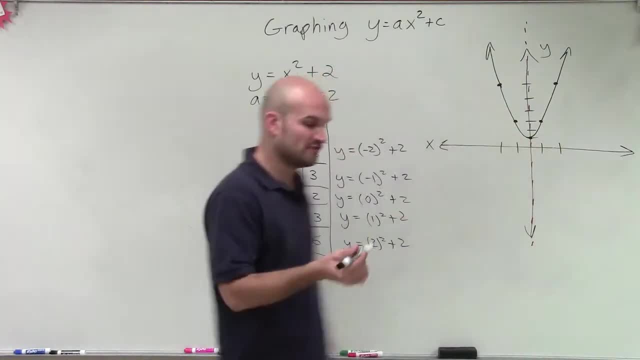 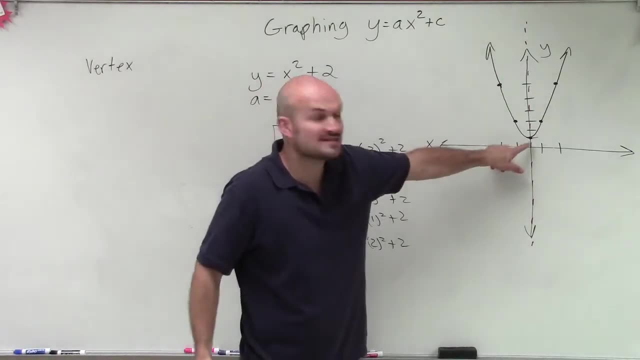 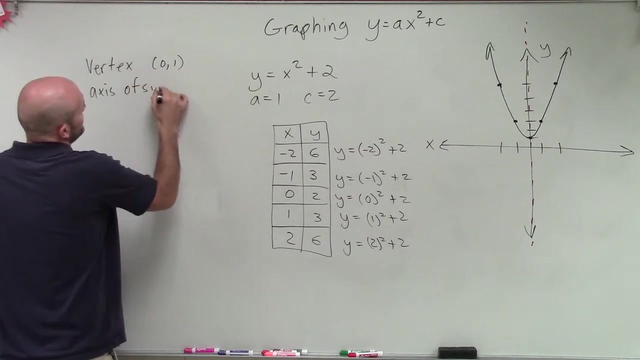 but it has a lower minimum point right there which we call our vertex. So when I want you to label the vertex, what I want to do is I want to label that exact point And we can see the vertex is a point at 0, 1.. The axis of symmetry which we've already talked about for all quadratics. 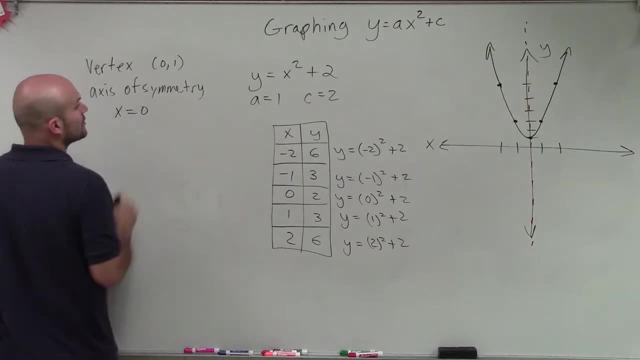 ax squared plus c is going to be x equals 0.. It's a vertical line in the form of x equals 0.. Now, when talking about the x-intercepts, we need to see where does the graph cross the x-axis? 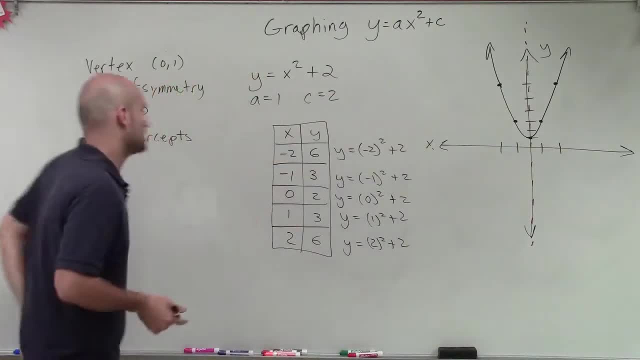 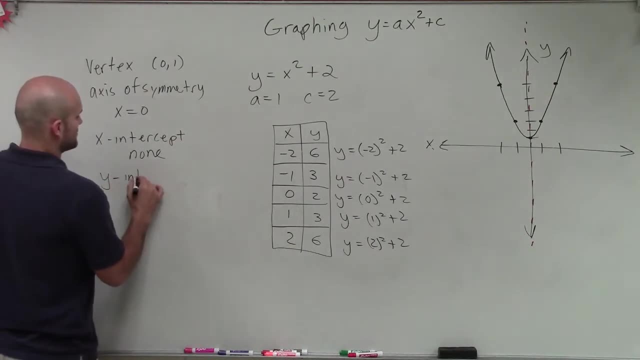 Well, you can see that this graph does not cross the x-axis, So we're going to talk a little bit more about that later. But we can just say there are none and it's only an x-intercept. And then we have y-intercepts. Actually, we're going to learn why they're going to be plural, Our y-intercepts. 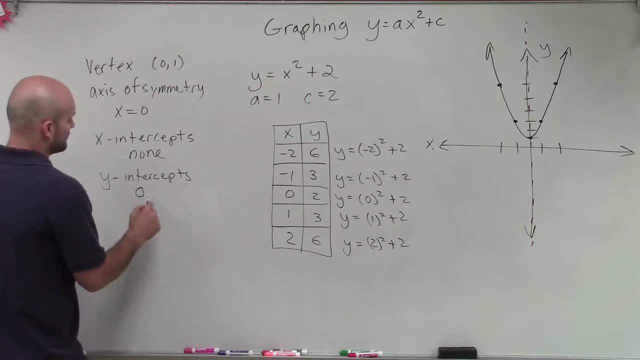 the graph classes at the y-axis at 0,, 1.. And that's at a point it crosses. So there you go, ladies and gentlemen. That is how you graph that equation. Thanks, 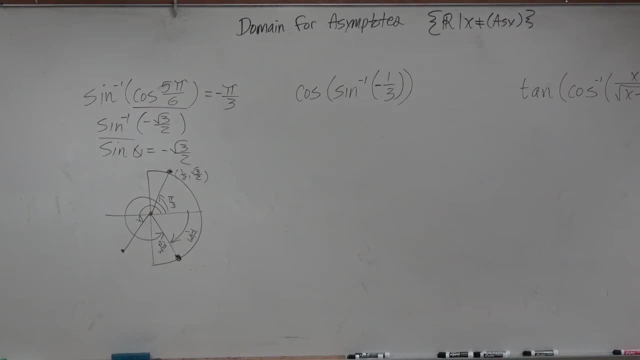 Think about this in terms of the unit circle, Because so far we just did a problem like this with the unit circle. So then I look at this and I say, OK, what angle gives me negative 1 third for sine? So I'm thinking of coordinate points, I'm thinking unit circle. 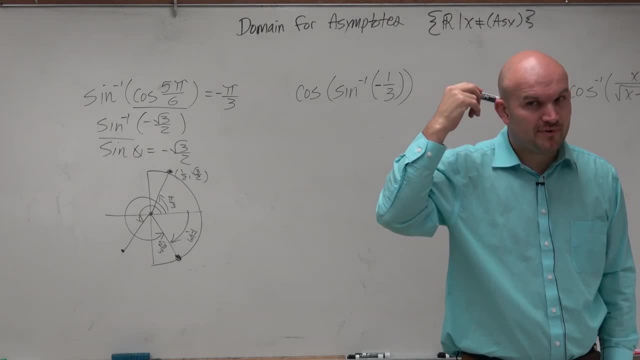 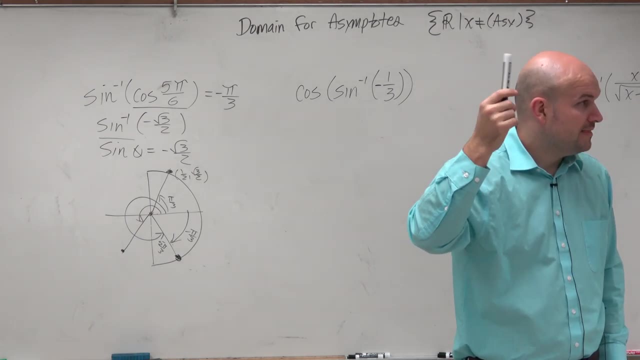 I just did this. I'm like, oh crap, I don't remember a point where the y-coordinate was negative 1 third on the unit circle Right. And there's a very good reason for that, Because the y-coordinate is not going to be equal to negative 1 third based on giving this value.